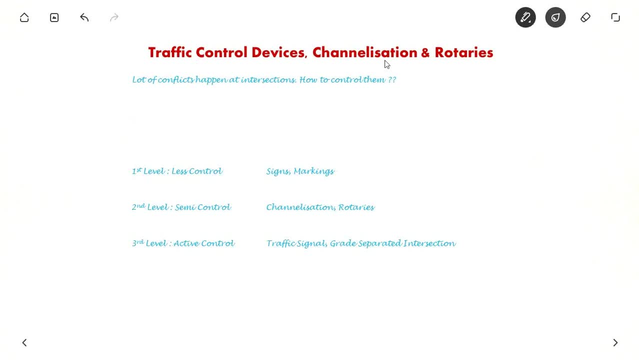 Hello everyone. In this video we will see about traffic control devices, channelization and rotaries. Often you observe that if there is an intersection there are lot of conflicts possible. So how to control these conflicts? For this only we have traffic control devices, channelization, rotaries, etc. So we can define them in three levels. First level is no controls, like leaving them uncontrolled. You can 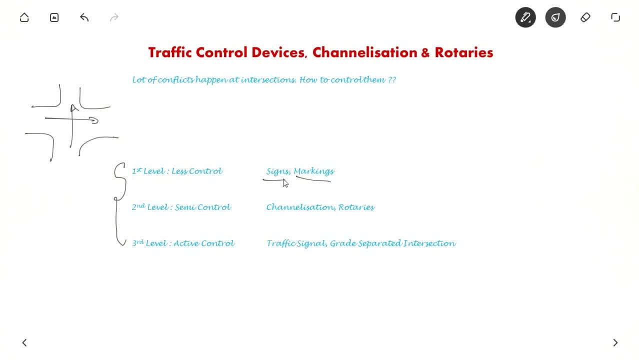 control little bit by signs and markings, by asking them to go slow or stop and go, conditions like that. Second level is semi control, little bit control by using channelization and rotaries. So this also we will see in the upcoming slides. And the third level is the highest level, which is using traffic signal. You ask them entirely to stop and you leave the other vehicles. 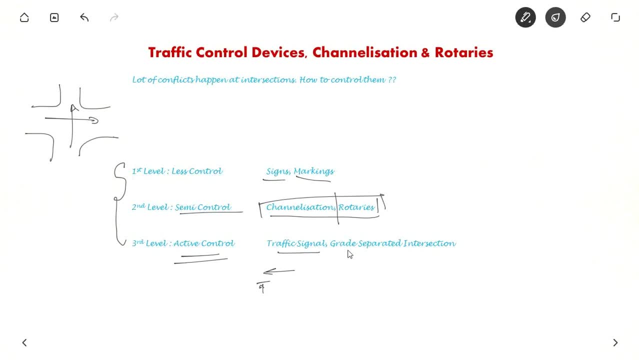 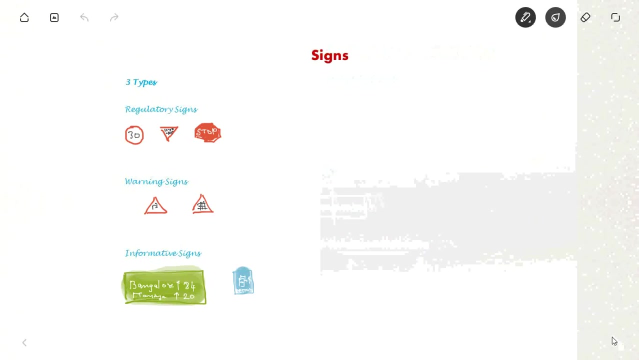 Then you ask these people to go. So that is active control. Another idea for active control is grade separated intersections. Suppose there are two roads passing like this. you provide a bridge, So that is grade separated. You are separating one grade from another grade. This is at a higher grade and this is at a lower grade. So that is grade separated intersection. Now we will see about signs. So there are three different types of signs. One is 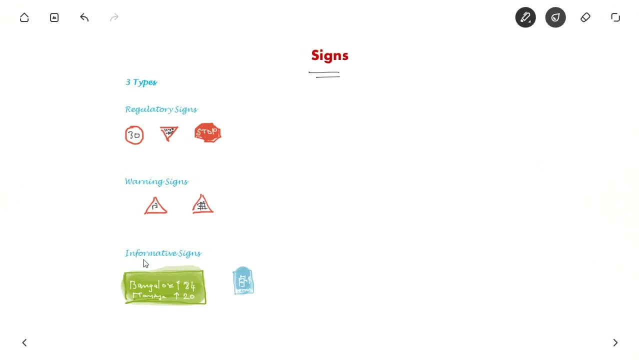 regulatory sign, another is warning sign and the third is informative sign. Regulatory signs are like speed limit or you can ask them to give way or stop. These two are used in intersections. Often you- not often- you- see a red border and a white background and the writing is in black. So this is usual for sign boards. 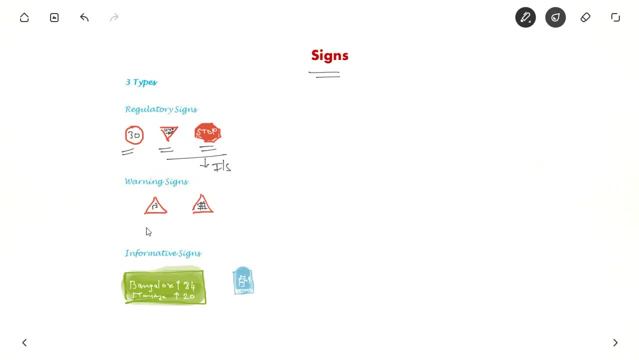 Warning signs. Warning signs are usually triangular in shapes. These are like caution signs The drivers may have to follow this. Regulatory signs are mandatory signs. So this is like right turn is approaching, or you say there is no right turn and you can warn them that a railway crossing is approaching. So these are warning signs. The third set is informative signs which provide information to you. 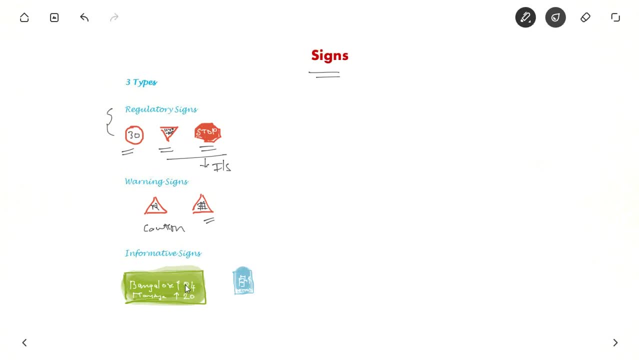 You may have observed while going to a different city how much distance is left. Usually it is given in a green board, And have you observed this? Petrol pump signs are blue in color. If you have observed this, please click yes here. Maybe you have observed while going to different places. So these are the three different types of signs which you need to know. 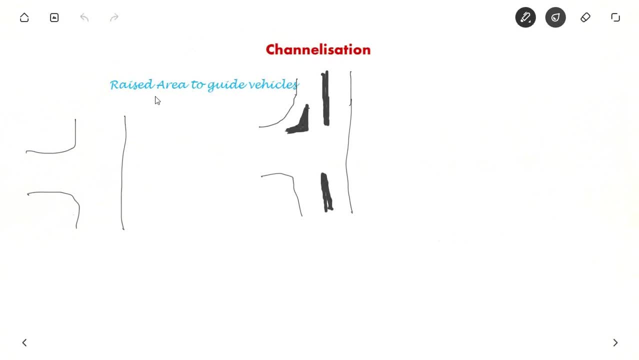 Channelization. Channelization is a raised area to guide the vehicles. Suppose this is a road without channelization, So one vehicle goes left here, Other vehicle through movement, So there is a conflict point here. So if you give a raised area to guide the vehicles the conflict area is reduced like this: So when you go left turn you follow a guide. 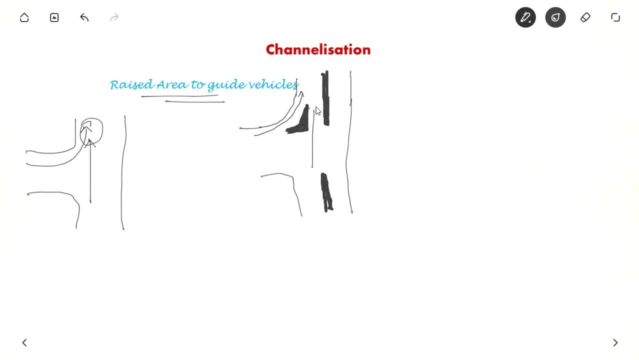 You follow a guided path like this, And through movement is like this. So the conflict area is reduced to a very small area. So that is why we have channelization Rotaries. The idea of a rotary is to convert the major conflicts into minor conflicts. Let us see how. So when you are coming for a through movement, you go like this: 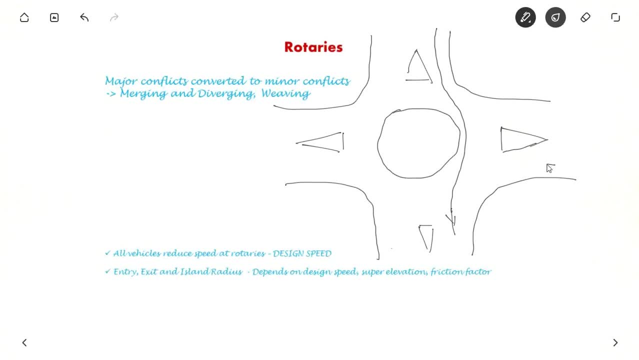 So you do positive and negative, And So this, through conflict, becomes a weaving conflict, And also when you have to go right from here, So here it becomes a merging conflict, And this is a diverging conflict. Every conflict is converted to merging, diverging and weaving conflict. reverse: 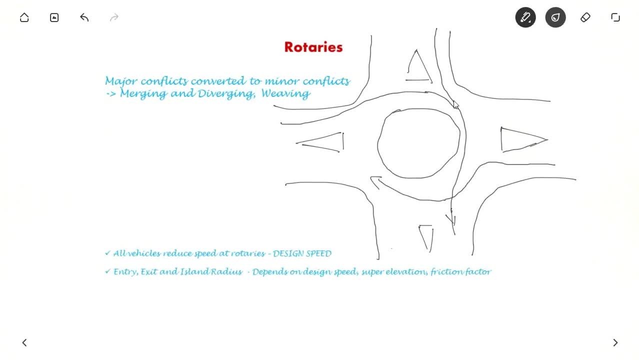 And therefore there is no conflict. So if you have Leuten will leave one road by circular route and remove hand говорил traffic, then you would have done two road at a distance, And so it should actually represent a diverging conflict and a divergingacks. 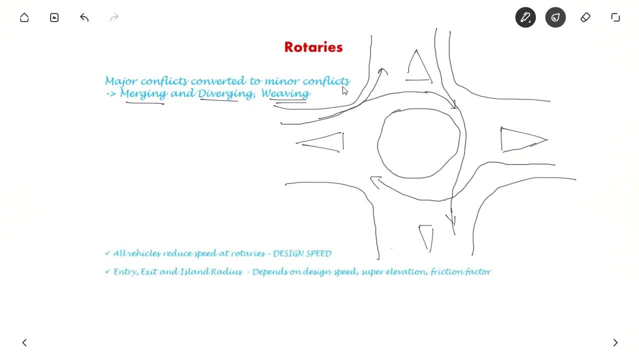 That cyber conflict will move around. two roads Go back, So the number of conflicts are minimized. that is the idea of a rotary. The terms of the rotary are: this is the central island, so this is the radius of a central island, and this is the entry radius and this is the exit radius, so radius is provided. so that the vehicles slow down while entering and while leaving. they will leave like this. The entry, exit and island radius depends on the design speed. Like, any vehicle which comes here reduces their speed, so that is the design speed for which the rotary is designed.